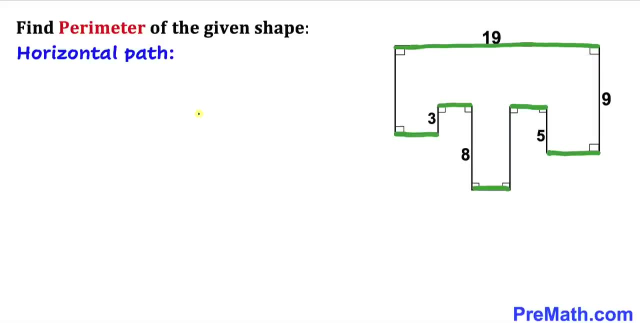 diagram. So, therefore, the total horizontal distance I'm going to represent h for horizontal distance- is going to be 19 plus 19, So our horizontal length turns out to be 38 units. And here's our next step. Let's go ahead and focus on the vertical path of this boundary. 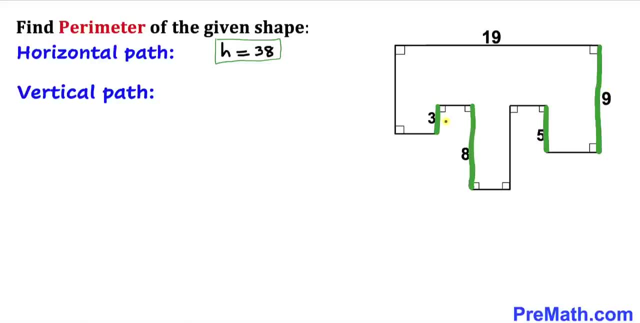 Now we know the value of these vertical segments. This is 3 units, this is 8, this is 5 and this is 9.. and This is 5 and this is 9.. going to calculate the vertical length of these segments, this one and this one as well. So, 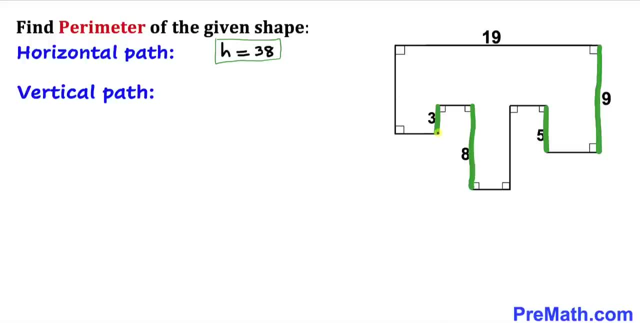 therefore, we are going to draw these dotted lines over here and likewise over here as well, and now we can see that this length is three units. so, therefore, this length is going to be three units as well. and now we know that this whole length is five units and we know this part is three. so 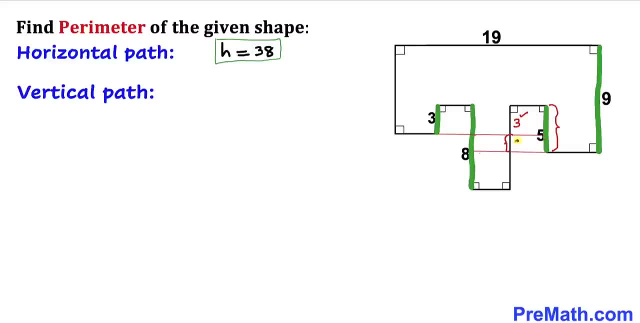 therefore this part is going to be two units, and now we know that this whole length, from here to here, is eight units. so therefore this whole length is going to be eight units as well, and now we know that these two individual lengths are five units. so therefore, the remaining this is going to 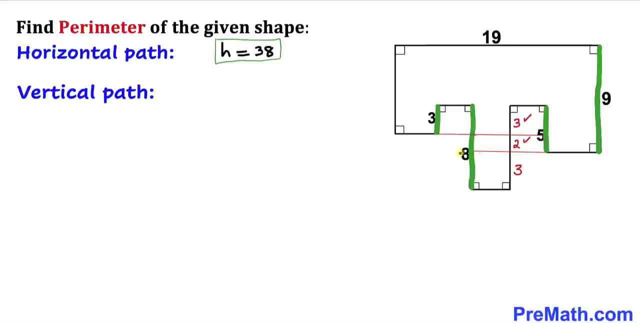 be three units as well, since they add up to eight units. and finally, let's focus on this vertical length. we want to find the value of this one. this length is equal to this length and this tiny length is equal to three units. so, therefore, this length has got to be nine minus two is going to be seven. 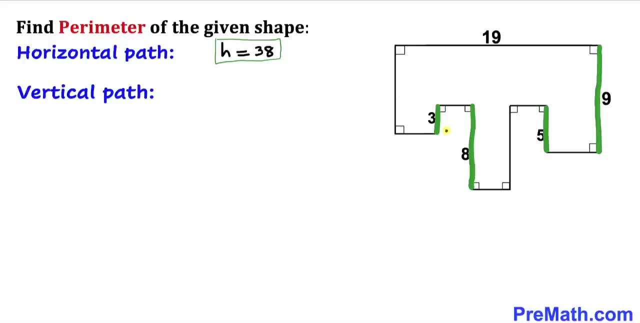 So, therefore, we are going to draw these dotted lines over here and likewise over here as well, And now we can see that this length is 3 units. so therefore, this length is going to be 3 units as well. And now we know that this whole length is 5 units and we know this part is 3, so therefore, this part is going to be 2 units. 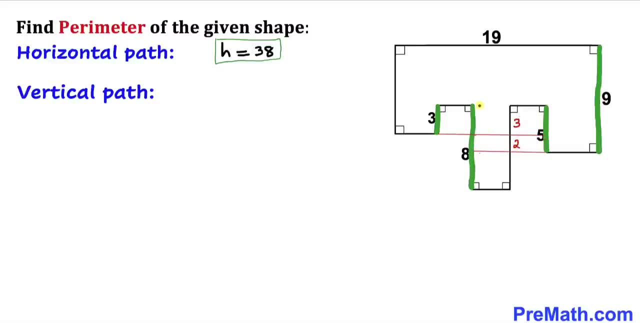 And now we know that this whole length, from here to here, is 8 units, so therefore this whole length is going to be 8 units as well. And now we know that these two individual lengths are 5 units, so therefore the remaining this is going to be 3 units as well, since they add up to 8 units. 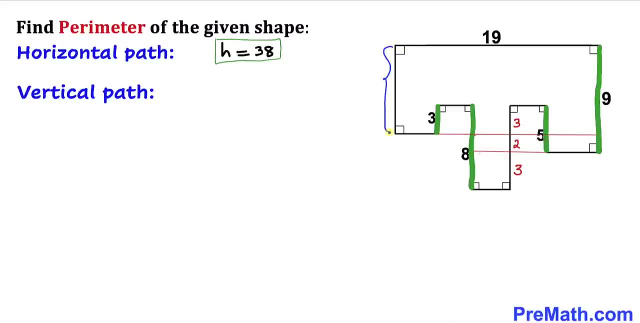 And finally, let's focus on this vertical length. We want to find the value of this one. This length is 8 units, This length is equal to this length And this tiny length is 2 units. So therefore, this length has got to be 9 minus 2 is going to be 7 units. 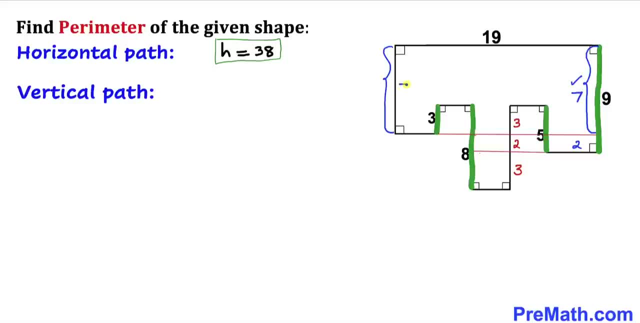 If this length is 7 units, then this vertical length is going to be 7 units as well. So, therefore, our total vertical path is going to be 7 units. So, therefore, vertical length is going to be 7 units And, as you can see, the vertical path is going to be 7 plus 3 plus 8, plus 3, plus 2 plus 3 plus 5 and, finally, plus 9 units. 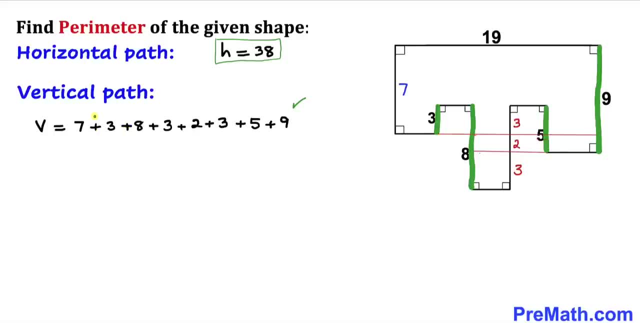 As you can see over here, we have added these numbers up and the�도. it represents the vertical path. Here you can see this: 7 is counted for this one. 3 is right here, right here. 8 is right here. all these 3, 2, 3 are right up here. finally, this is 5.